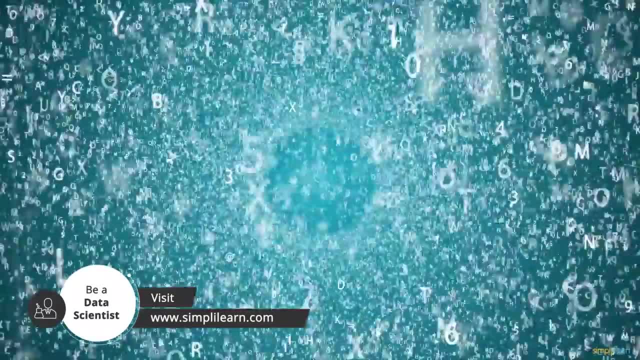 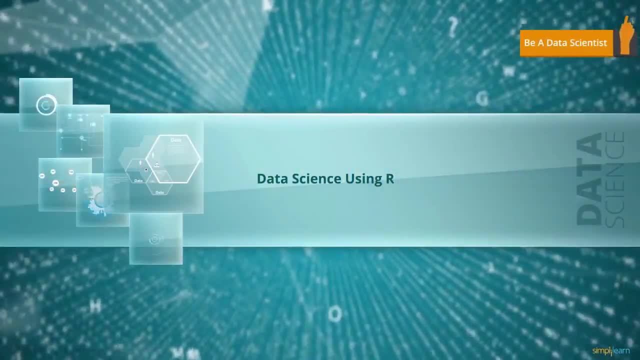 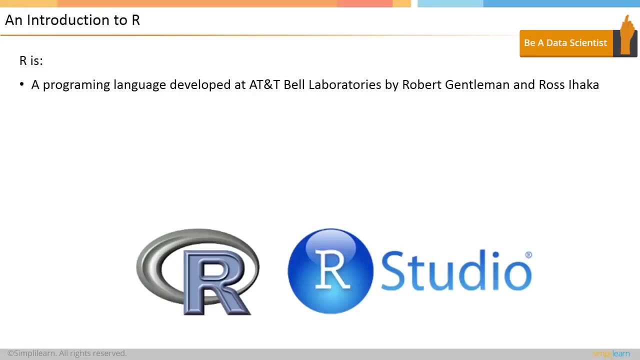 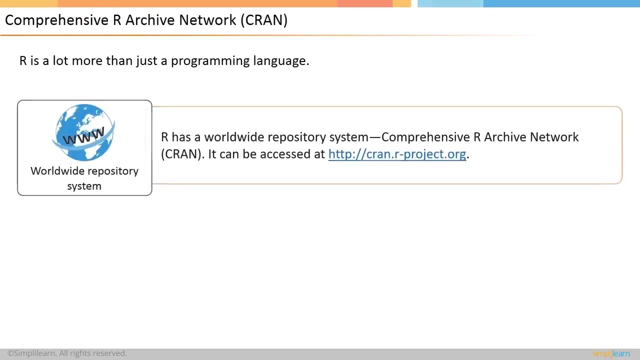 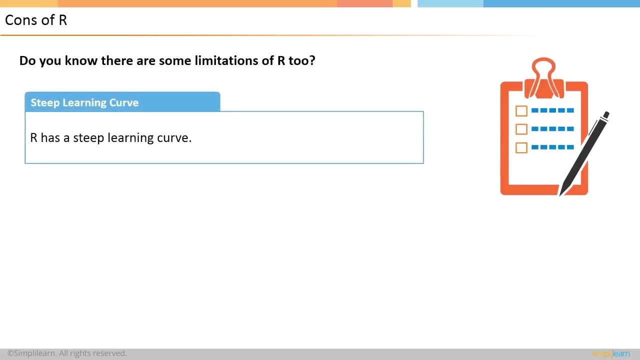 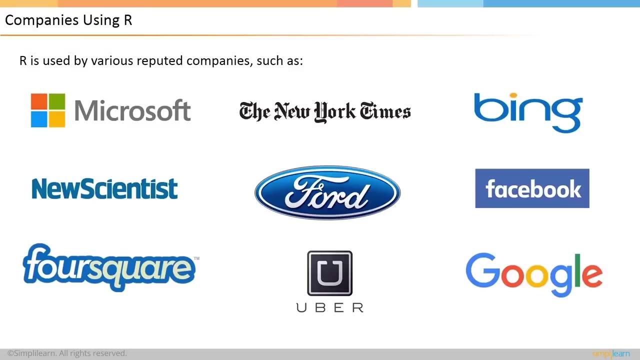 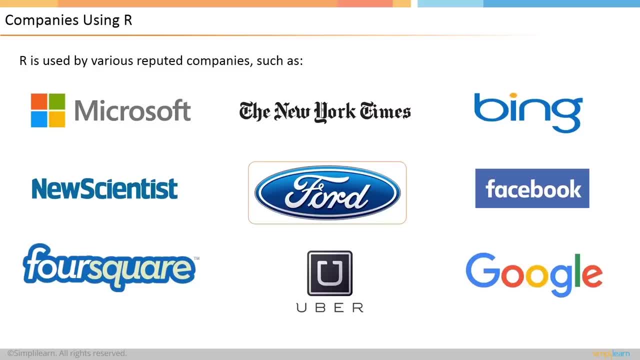 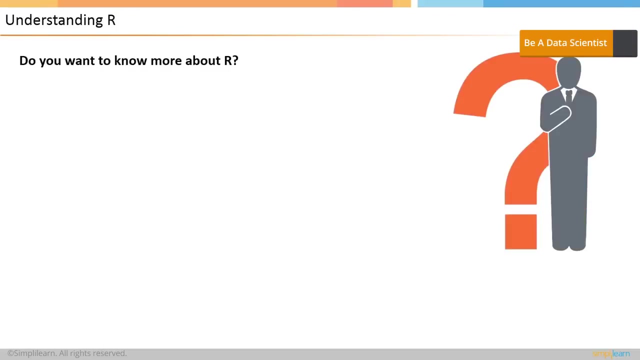 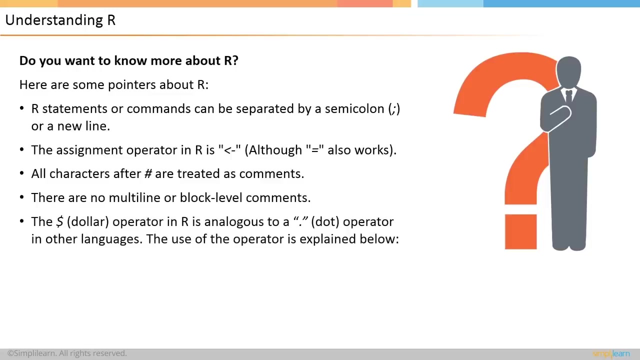 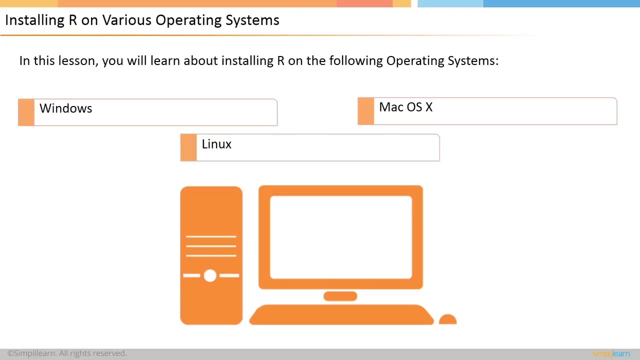 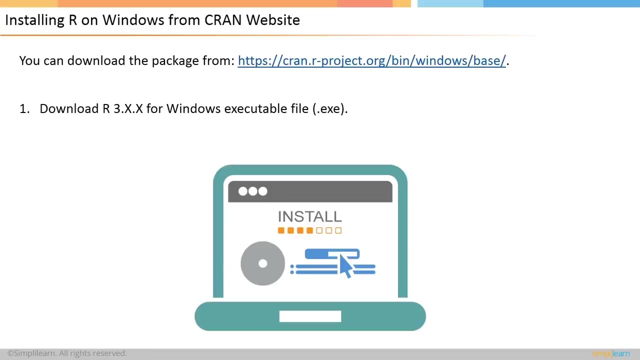 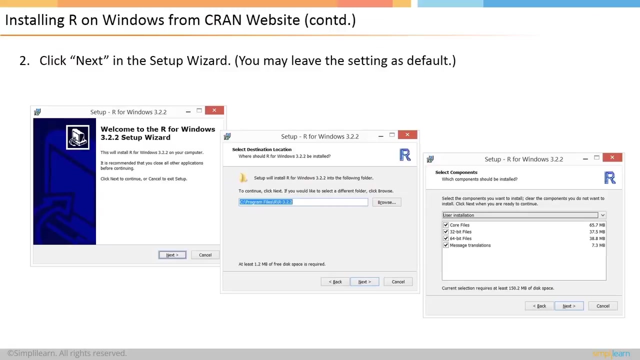 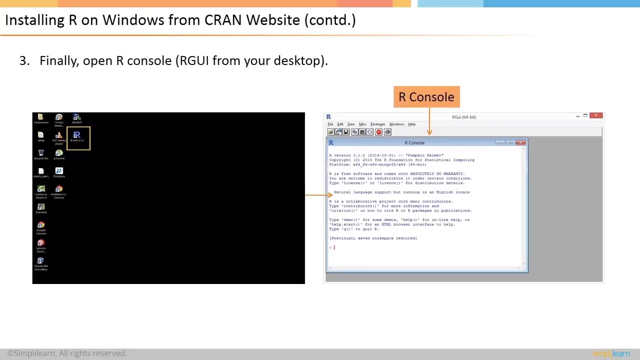 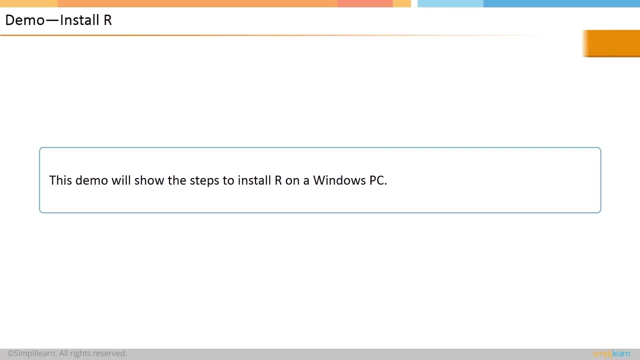 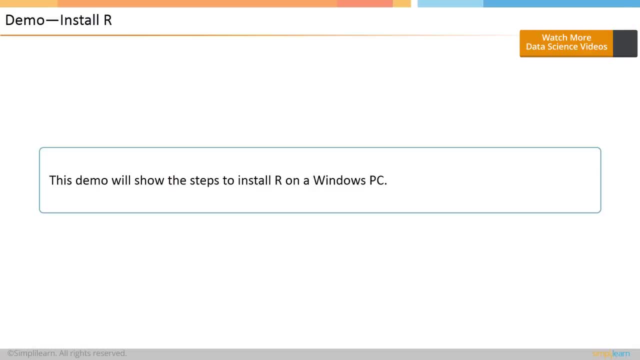 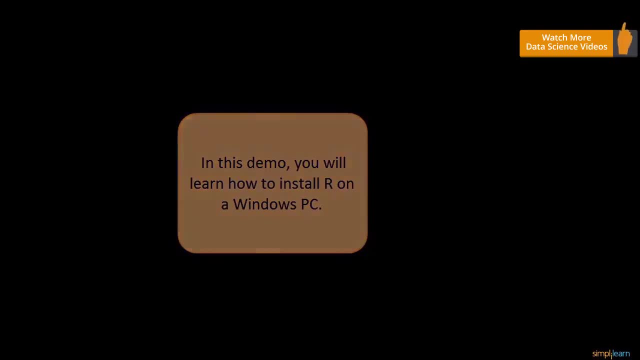 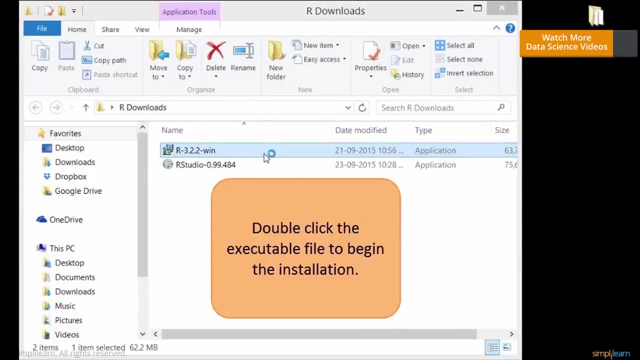 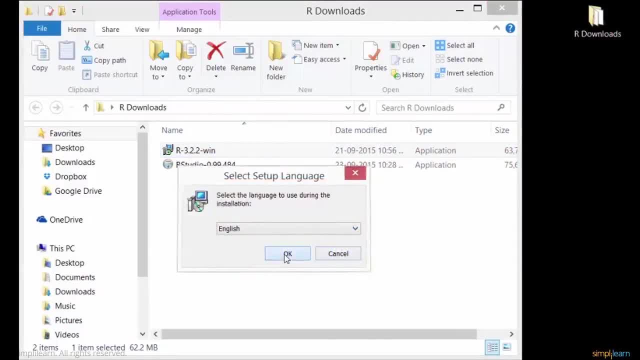 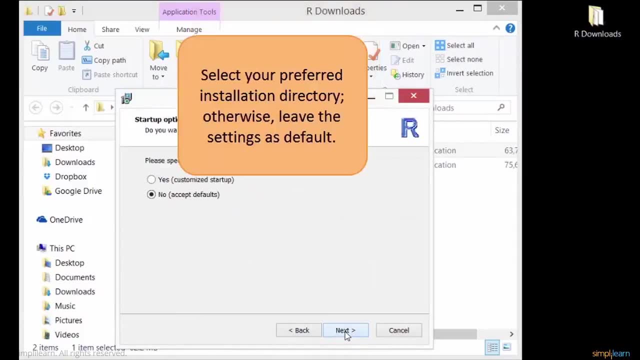 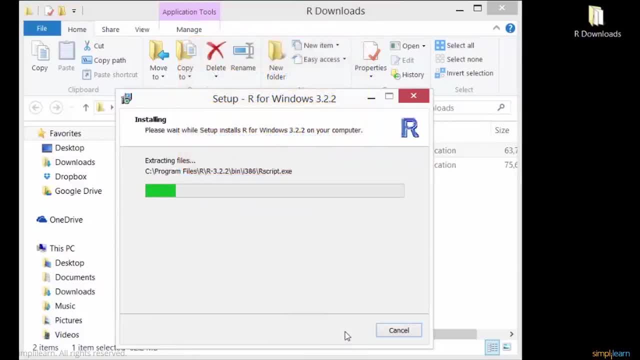 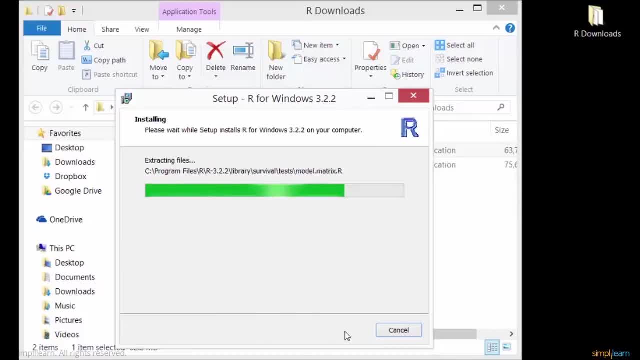 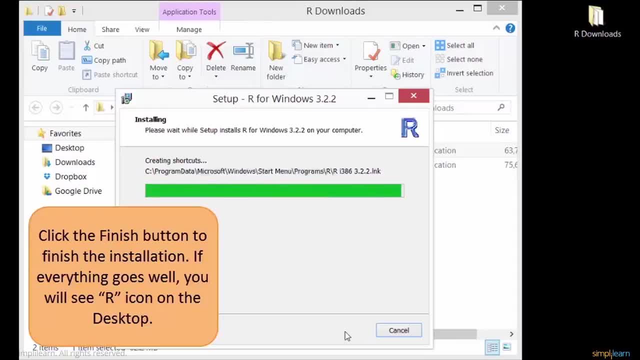 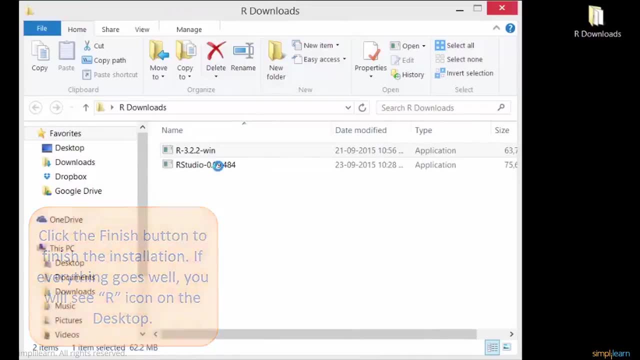 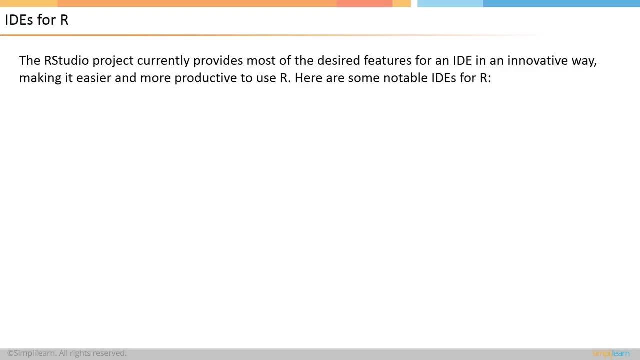 Transcription by: — Click the Finish button to finish the installation. If everything goes well, you will see the R icon on the desktop. RStudio is an IDE or Integrated Development Environment for R. It's a project that provides most of the desired features for an IDE in an innovative way, which makes it 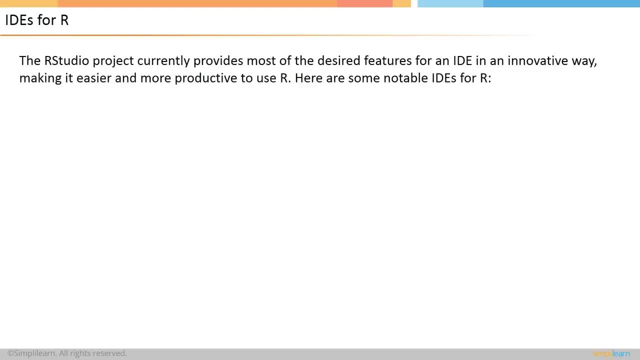 easier and more productive to use R. It includes a console and tools for history plotting, workspace and debugging management. It also includes an editor that highlights the syntaxes, which supports execution of the code directly. Some other notable IDEs are listed in the table shown on the screen, along with the 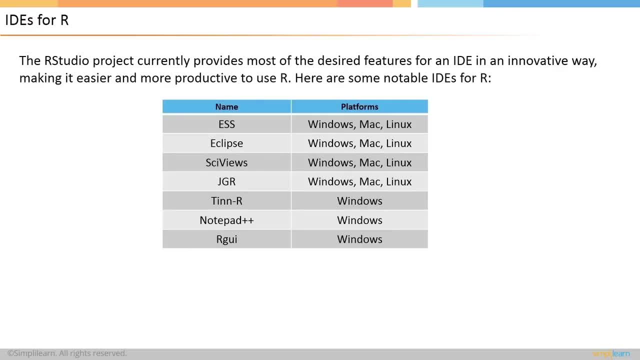 supported platforms. RStudio is available in various commercial and open-source editions. It can be run on a desktop or through a web browser connected to RStudio Server or RStudio Server Pro. The desktop version is available for Windows, Mac OS X and Linux. 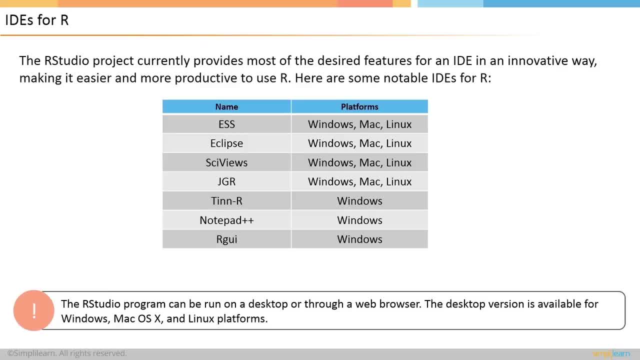 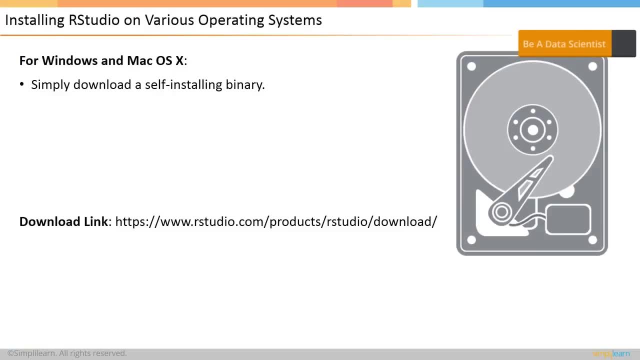 To install RStudio on a Windows or Mac OS X system, you would need to simply download its self-installing binary. For this, you would need to go to the RStudio official website given on the screen and download the appropriate version for your system. 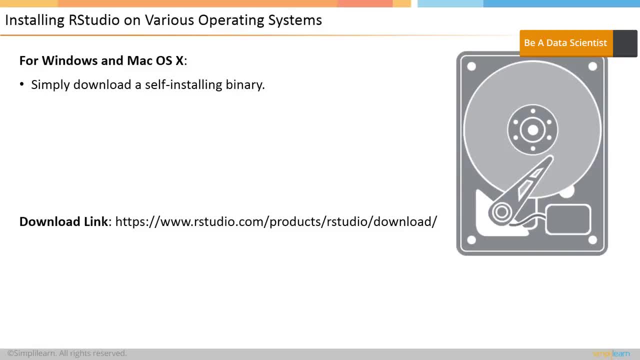 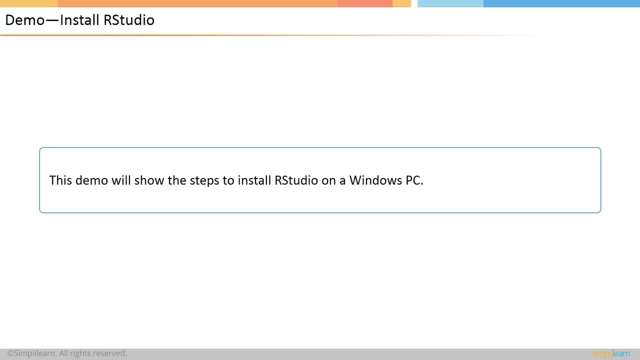 Next you would need to double-click the downloaded executable file and start the installation process. However, for Linux, the installation process varies. For Debian Distribution, including Ubuntu, you can install the RStudio using its regular package management tools. This demo will show the steps to install RStudio on a Windows PC. 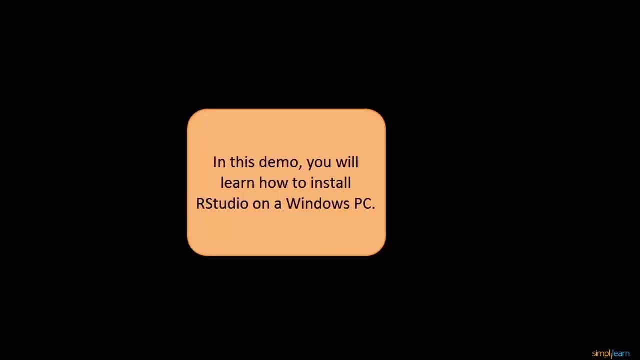 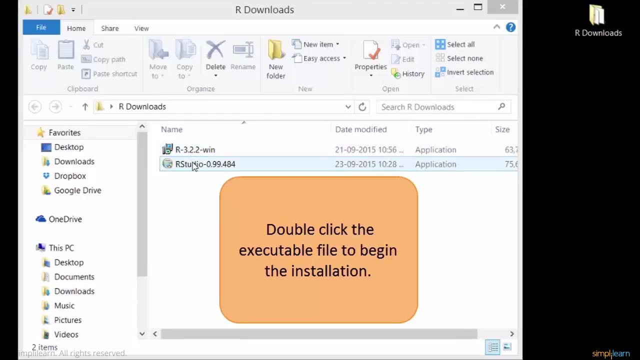 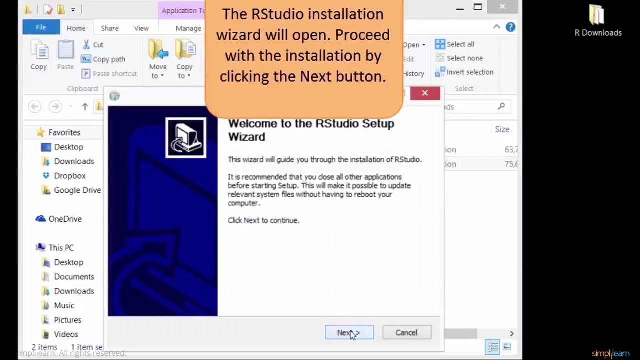 In this demo you will learn how to install RStudio on a Windows PC. Download the latest Windows RStudio package from the given URL. double-click the executable file to begin the installation. Then download RStudio for your Windows PC. The RStudio installation wizard will open. 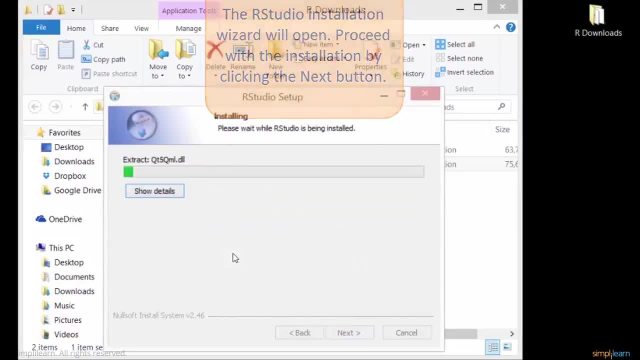 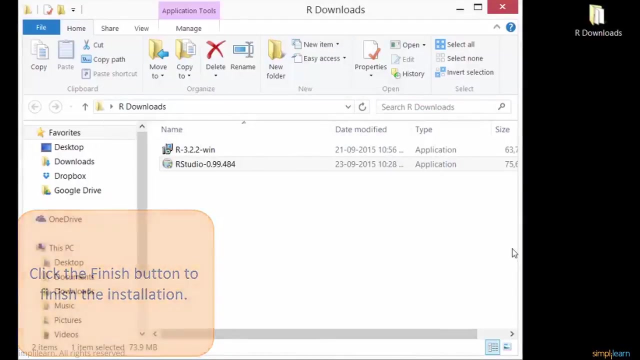 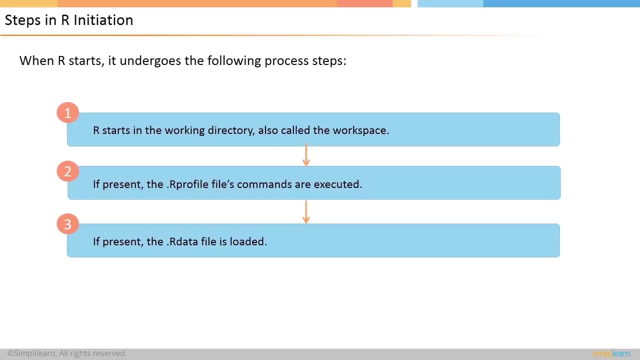 Proceed with the installation by clicking the Next button. Select your preferred installation directory. otherwise leave the settings as default. Click the Finish button to finish the installation. When R starts, it undergoes the process steps as shown on the screen. It starts in the working directory, which is also called the workspace. 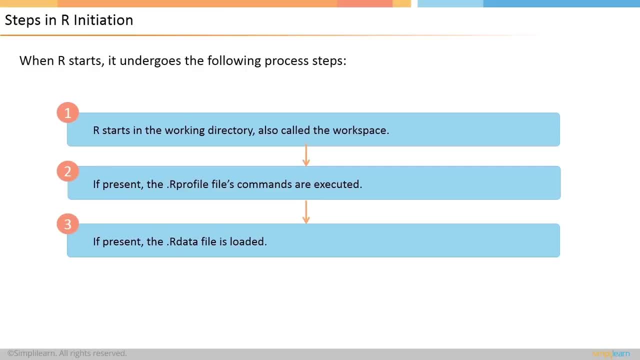 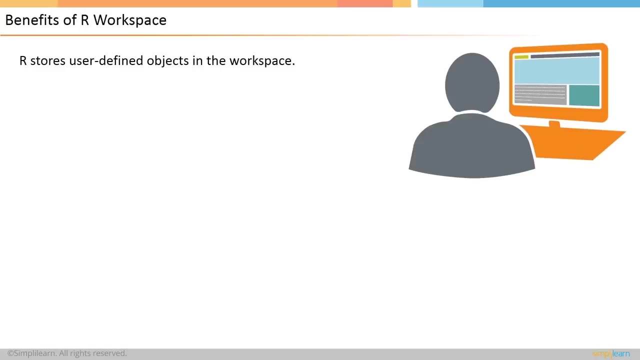 The rprofilefiles commands are executed next, if they are present At the end. if present, the rdata file is loaded. The R workspace is the current working environment of R. It includes user-defined objects such as matrices, lists, data frames, functions and vectors. 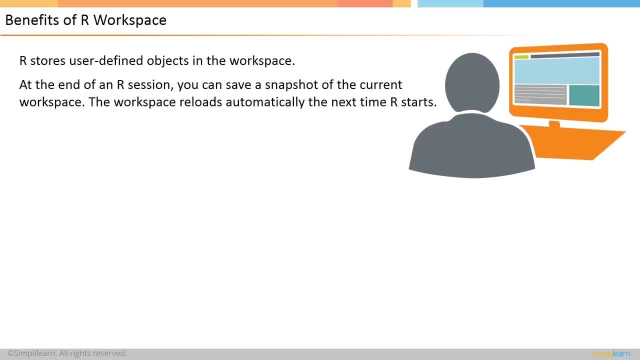 At the end of an R session you can save a snapshot of the current workspace. The workspace reloads automatically the next time R starts. In this you can enter commands interactively at the R user prompt. You can also use up and down arrow keys to browse through your command history. 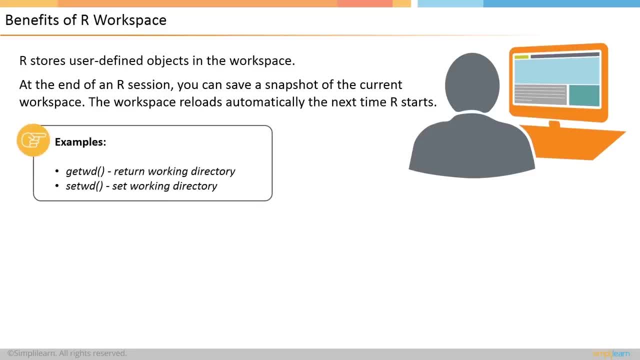 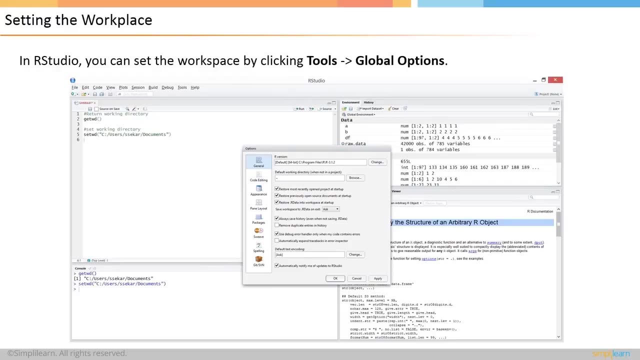 Here are a few examples of such commands: Get WD is the command that prints the current working directory, and set WD is the command that sets the working directory To set the workspace in R Studio you can click Tools and then Global Options, as shown on the screen. 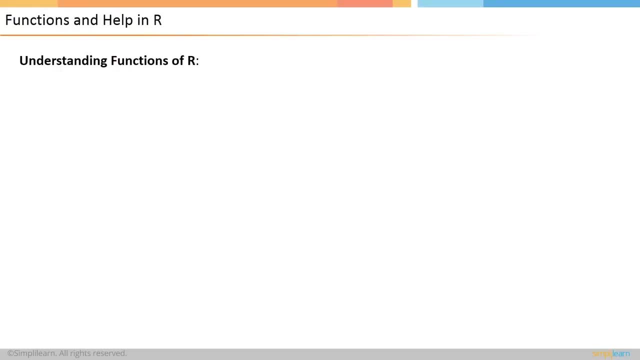 R has many functions that can be used to perform sophisticated tasks. At the core, it has above 1,000 functions. In addition, several new ones are created all the time. At the core, it has above 1,000 functions. 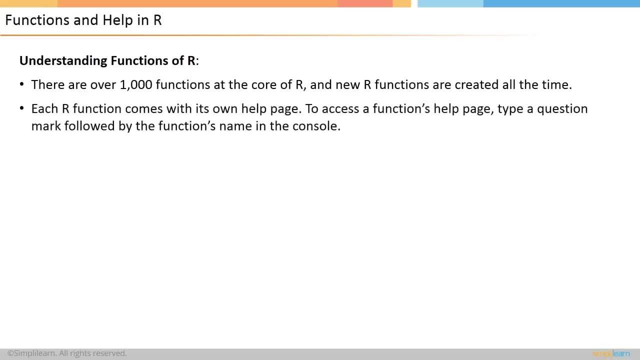 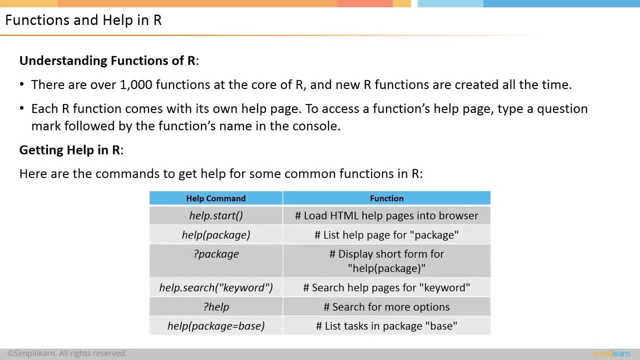 In addition, several new ones are created all the time- has its own help page. To access the same, you can type the name of the function in the console, preceded by a question mark. The table given on the screen shows the commands to get help for some common functions in R. 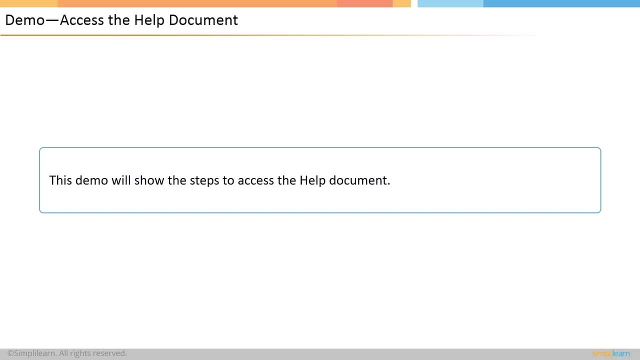 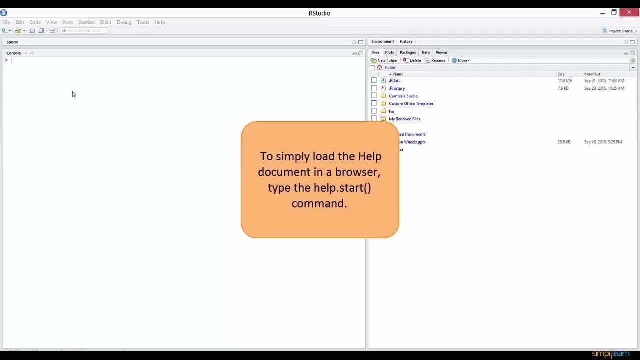 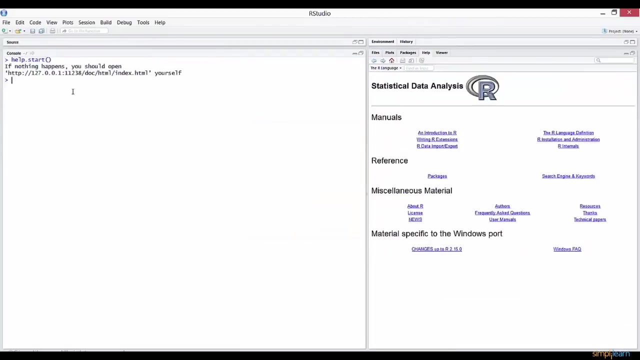 This demo will show the steps to access the help document. In this demo, you'll learn how to access the help document. To simply load the help document in a browser type: the given command. To access the help document for a particular package type: the given commands. 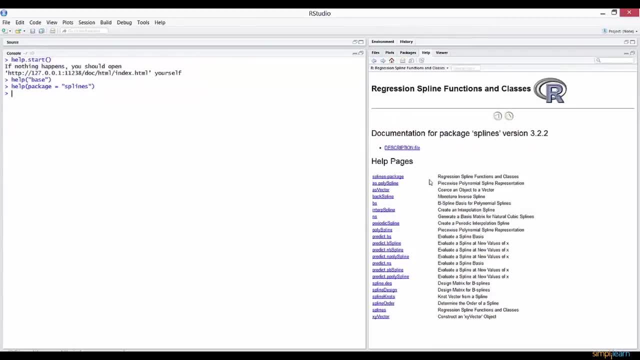 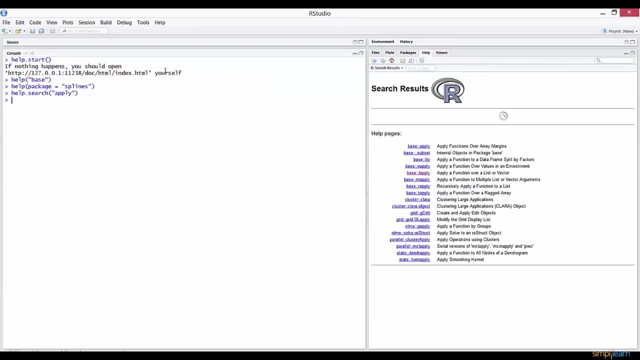 To access the search help document by keyword type: the given command. To access the search help document by keyword type: the given command. For more help options, try using the name of functions or package prefixed with a question mark. A few examples are given and some are not. 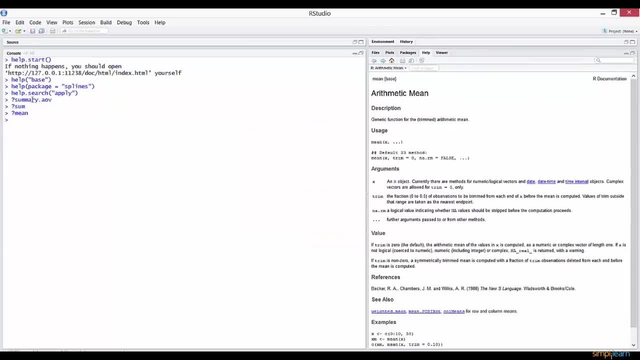 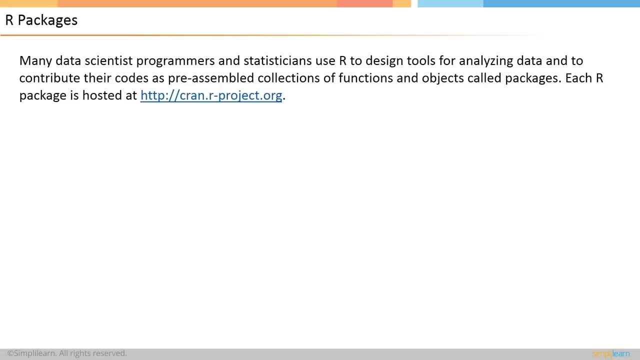 I'll show you a few here. Many data scientists, programmers and statisticians use R to design tools for analyzing data and to contribute their codes as pre-assembled collections of functions and objects called packages, and to contribute their codes as pre-assembled collections of functions and objects called packages. 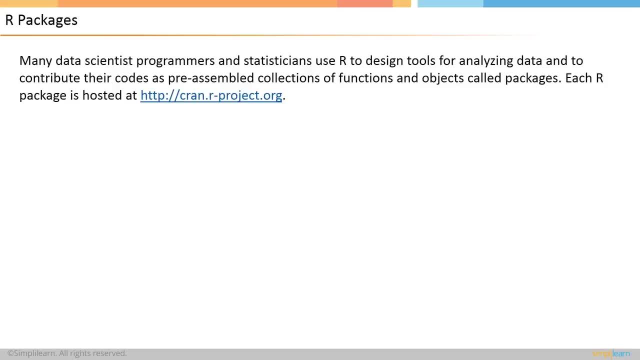 R packages are defined as collections of data, R functions and compiled data. These packages are stored in a directory called library. All these packages are hosted at the given page given URL. R includes a set of standard packages, while there are a few others that can be downloaded. 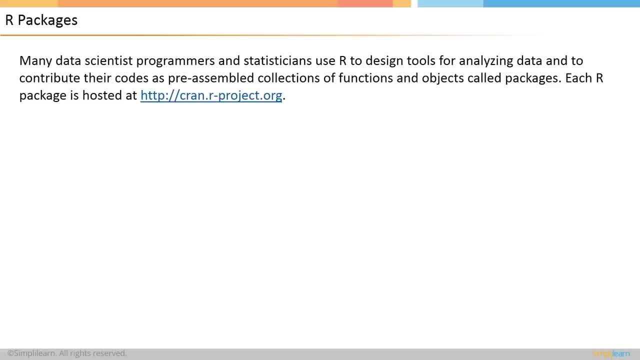 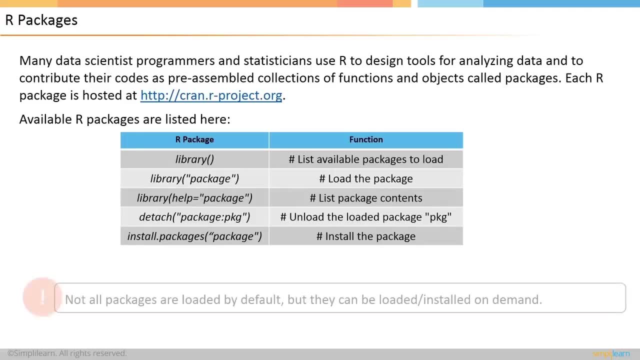 and installed. To use them, you would have to load them into a session. Some of the available R packages and their functions are listed in the given table. Note that not all packages are loaded by default, but they can be loaded or installed on demand. 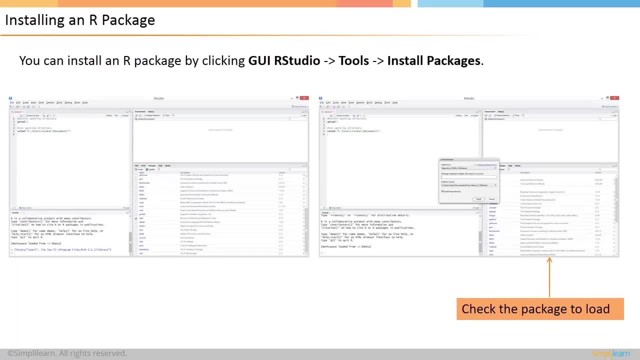 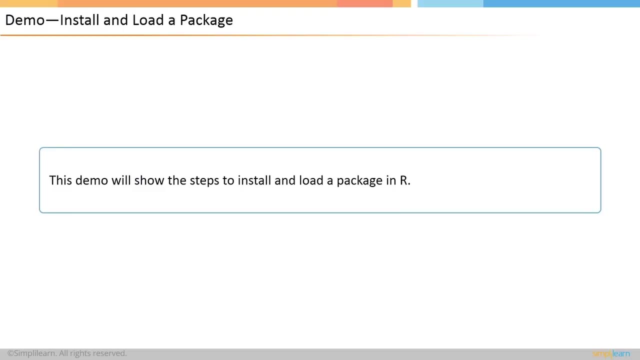 You can install an R package by clicking GUI RStudio Tools and then Install Packages as shown on the screen. This demo will show the steps to install and load a package in R. In this demo, you'll learn how to install and load a package in R.